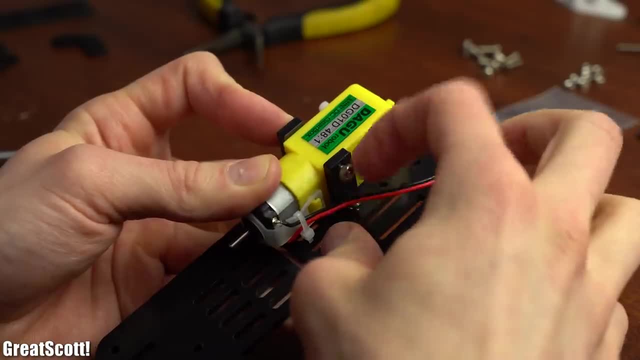 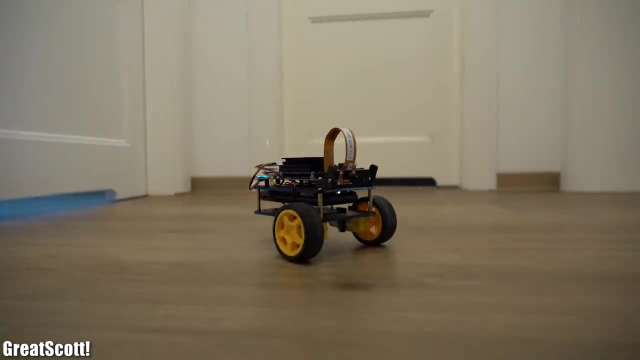 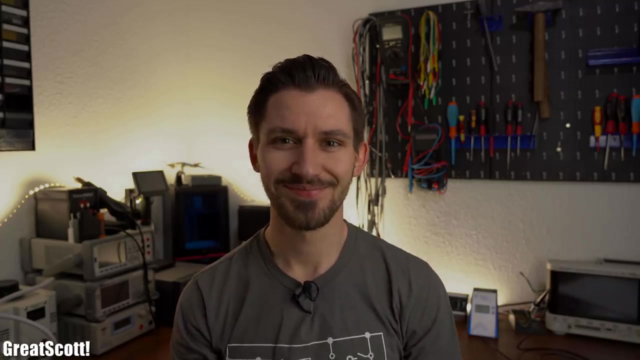 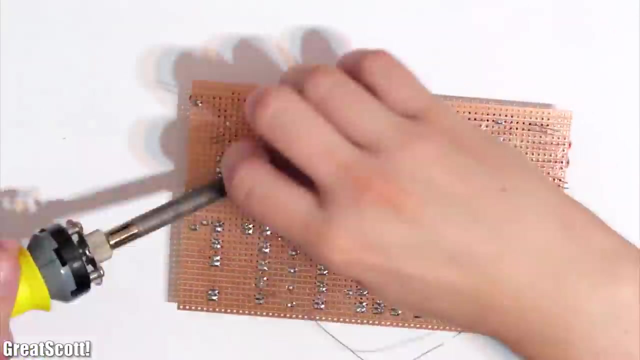 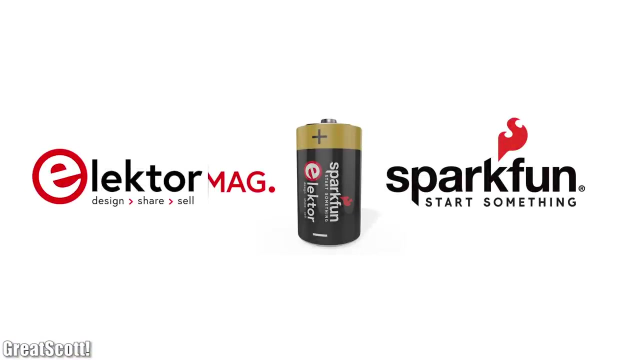 adventure together in which I will show you how I built a small robot that I trained, with around 600 pictures I've taken with it in order to let it drive around autonomously in my corridor without hitting any objects. Let's get started. This video is sponsored by Elektor and Sparkfun, who released a special edition of Elektor Mac three days ago. 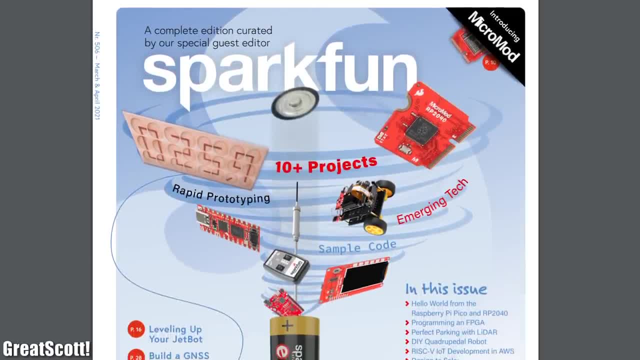 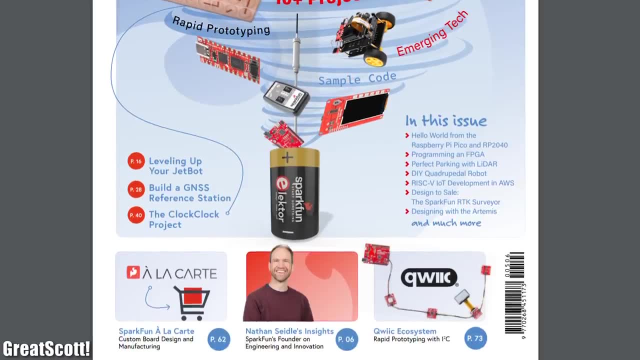 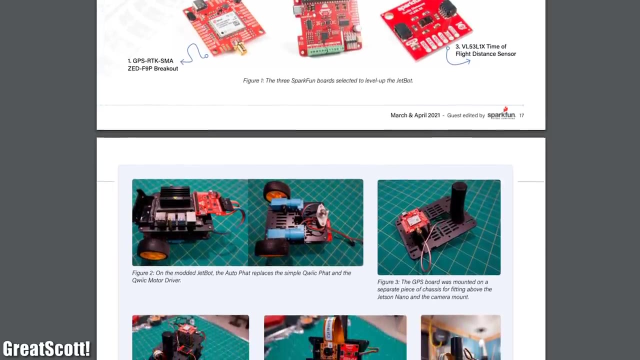 This edition is the result of a secret, creative collaboration between them. That is why Elektor is offering my viewers a 20% discount on a print copy and 50% discount on a digital copy of the new magazine, Which features exciting DIY electronics projects and engineering tutorials. 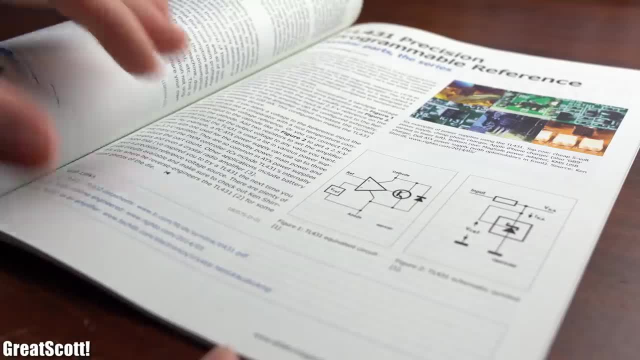 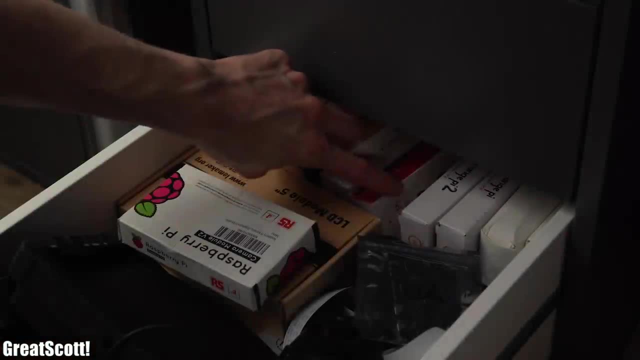 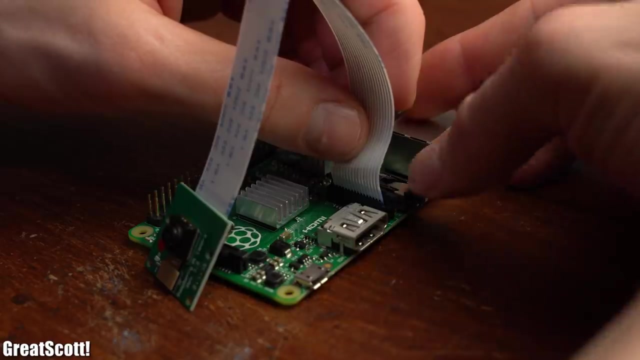 Check out the links in the video description to grab your discounted copy of this collector's item and see what more they have to offer. First off, we need some kind of small and powerful computer And yes, using a Raspberry Pi was also one of my first ideas, but I quickly learned through. for example, 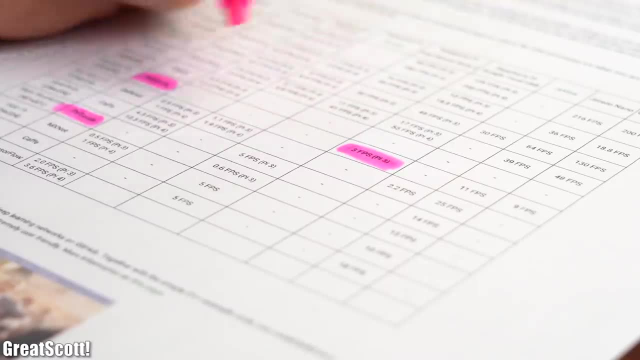 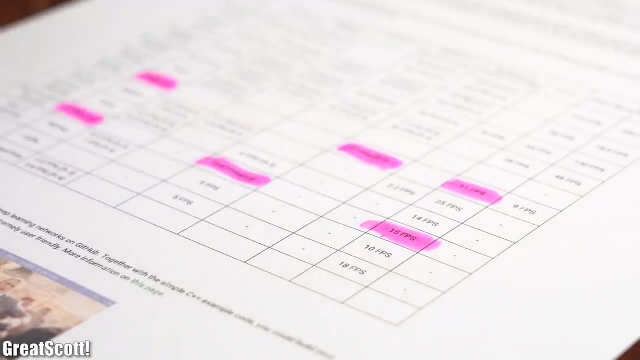 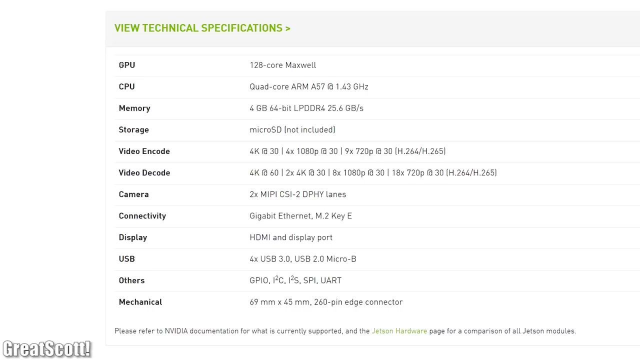 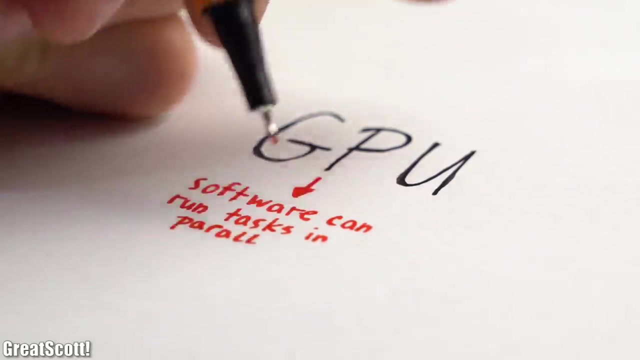 stuff created by Q-Engineering, that it apparently was not powerful enough for deep learning tasks. A single board computer that achieved useful results, however, was the Jetson Nano manufactured by Nvidia. The reason is that it comes with a way more powerful graphical processing unit, or GPU, which the AI or deep learning software can use to run tasks in parallel. 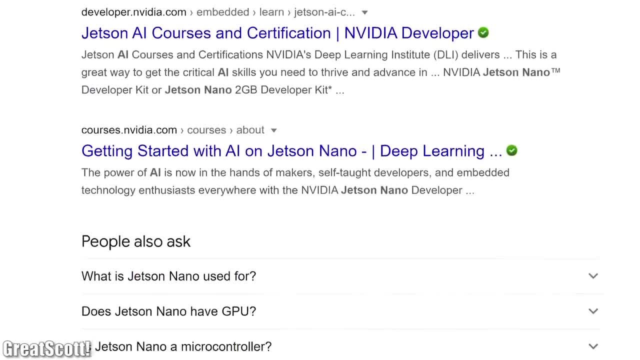 And while researching the software, I found that it was not powerful enough for deep learning tasks. The reason is that it comes with a way more powerful graphical processing unit, or GPU, which the AI or deep learning software can use to run tasks in parallel. And while researching this development board I've never worked with before- 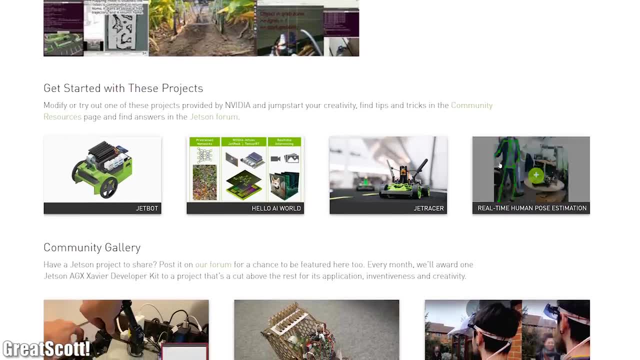 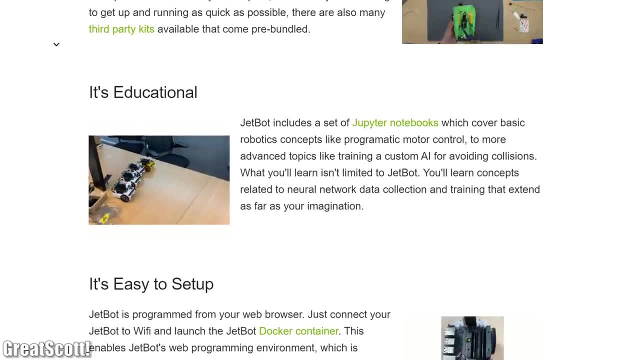 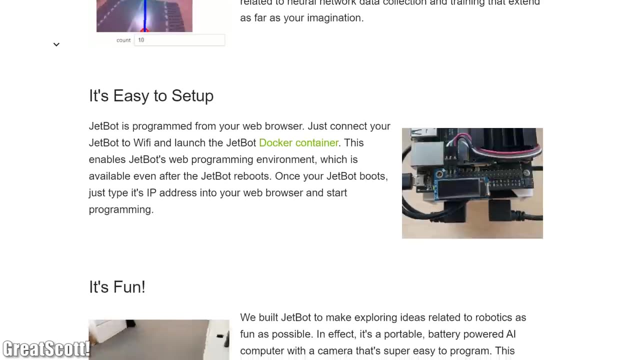 I realized that there already exists a project based around it, which is called the JetBot. It basically combines the computer with a camera, motor driver plus motors, OLED display and a chassis to create an AI robot, Which is just what I was looking for. 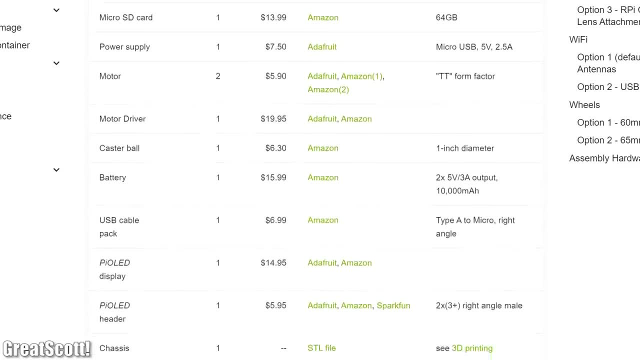 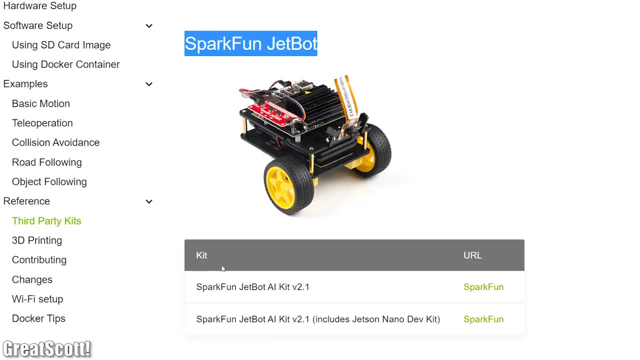 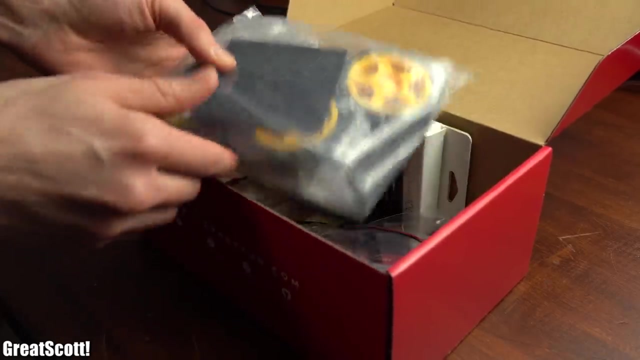 Now, of course, you could order the components for this robot by yourself And then 3D print the chassis, but I went with the simpler routes by simply getting a pre-made kit from Sparkfun. The really handy thing is that you not only get all components necessary for such an AI robot. 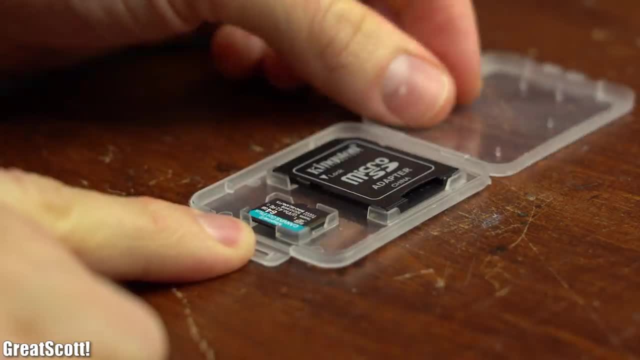 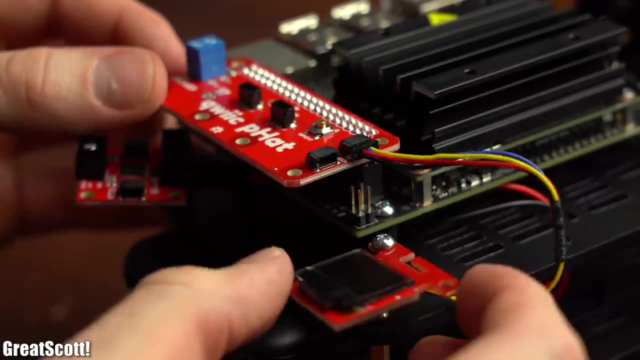 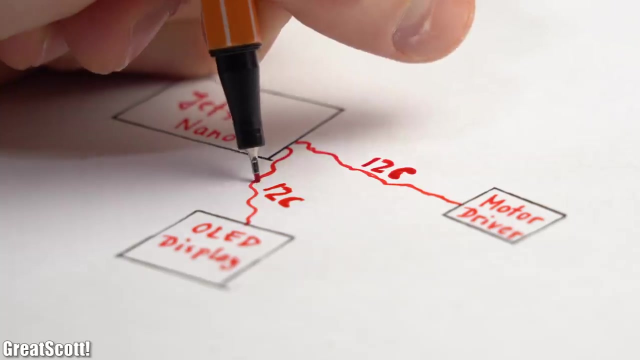 build this way, but you also get a pre-flashed micro SD card which comes with all of the software installed as well as all configurations for the hardware. This is important, since the hardware components use I2C And that can be a bit tricky to configure for beginners. 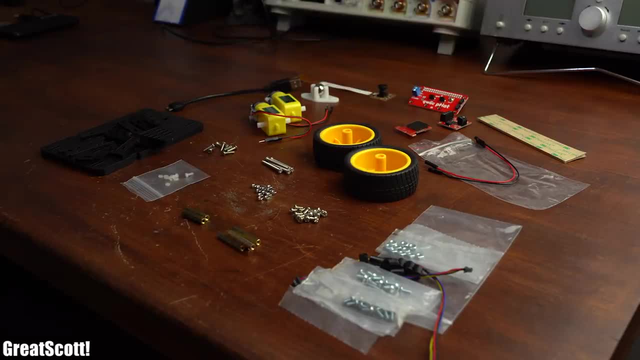 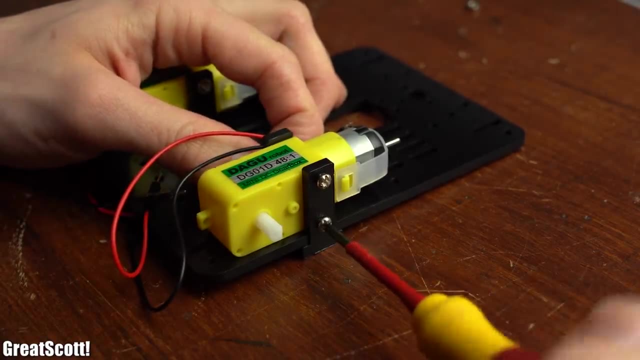 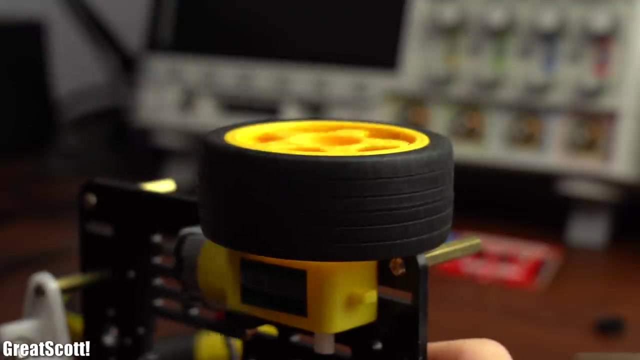 But anyway, with all the components in my hands, I had a look at the assembly guide on the Sparkfun website and started, like described, by attaching the motors to one base plate, After then adding several standoffs, the caster ball and the wheels. I already had the parts of the robot completed that could drive around. 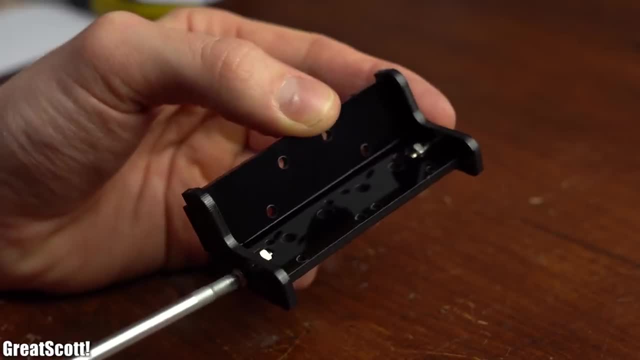 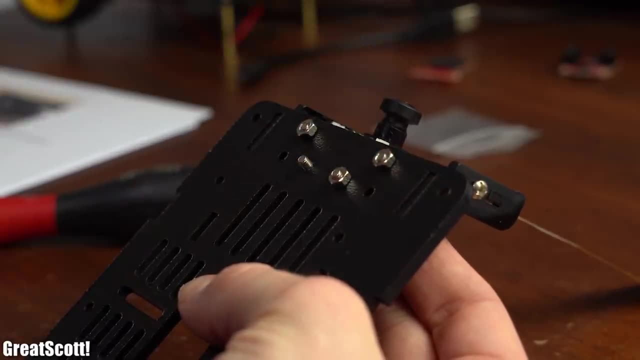 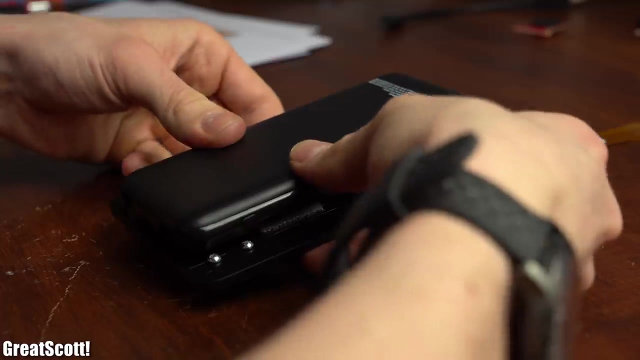 So I continued by assembling the camera holder, to which I obviously secured the camera before I mounted it all to the other base plate. Then I added more standoffs as well as the given power bank through the help of kind of velcro tape, combined the upper and lower base plate and mounted the motor driver before I finally 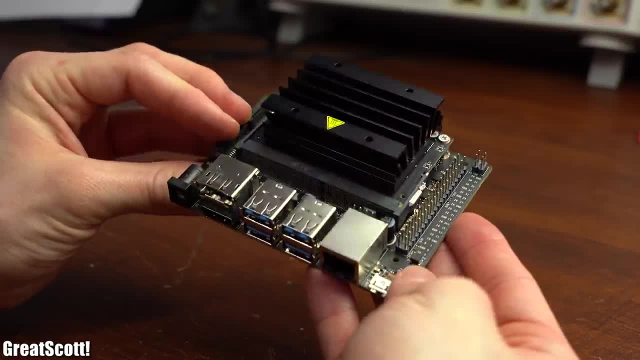 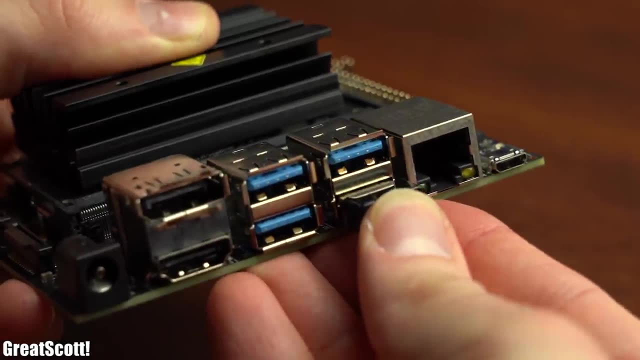 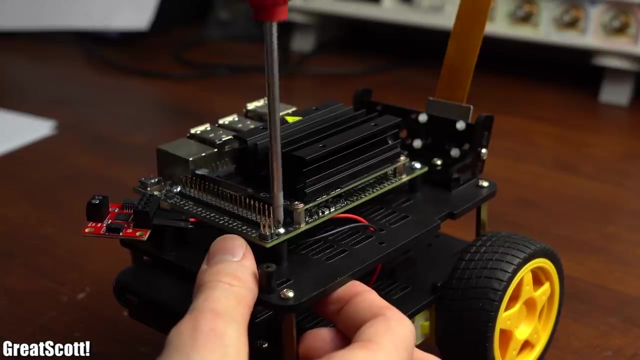 unpacked the Jetson single board computer And I have to say that it looked rather promising, So I added a WiFi Bluetooth dongle to it and inserted the given SD card before I mounted it on top of the robot. After then connecting the camera to it, I screwed the OLED display in place. 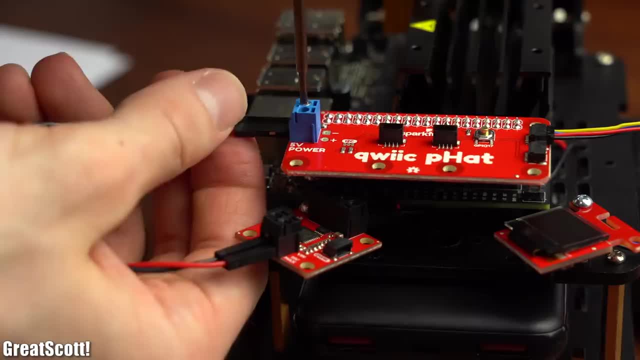 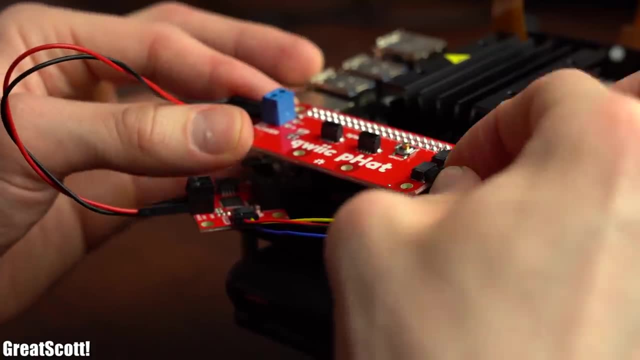 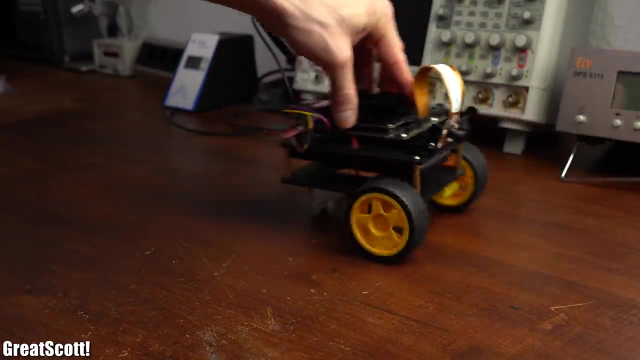 and pushed a breakout board onto the SPC, which I used to not only power the motor driver but also to connect all the devices to one another through their I2C data lines. And just like that, after around 2 hours of assembly, I got my AI robot. 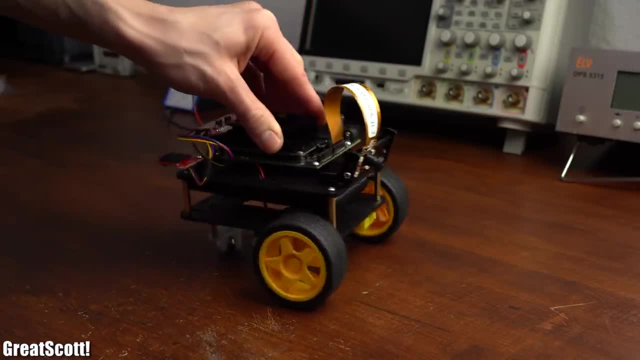 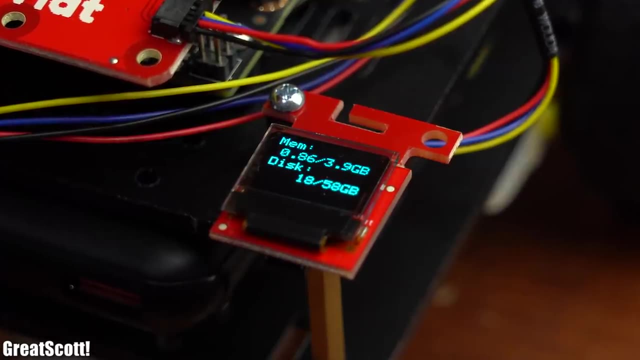 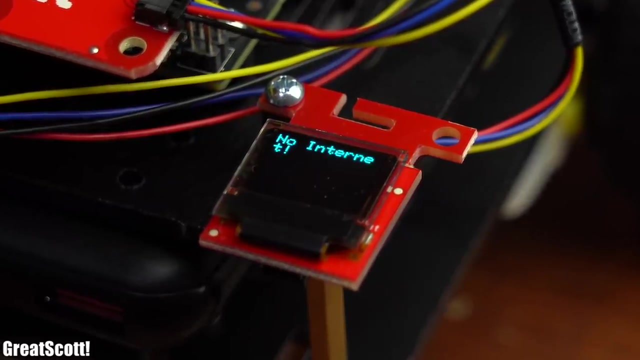 But of course the AI part was still missing. So I powered the computer through the power bank and after a few minutes the OLED display told me that the system was not connected to the internet. Who would have thought To solve that? I connected a small display, along with keyboard and mouse, to the computer. 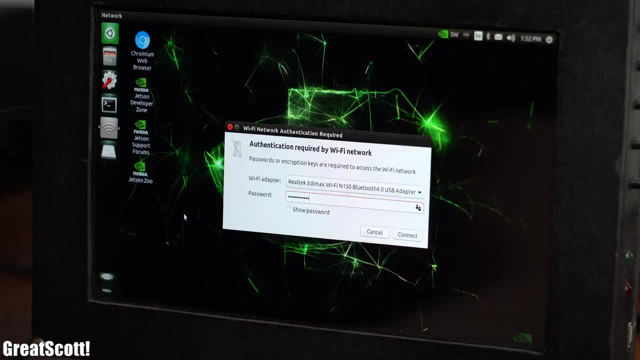 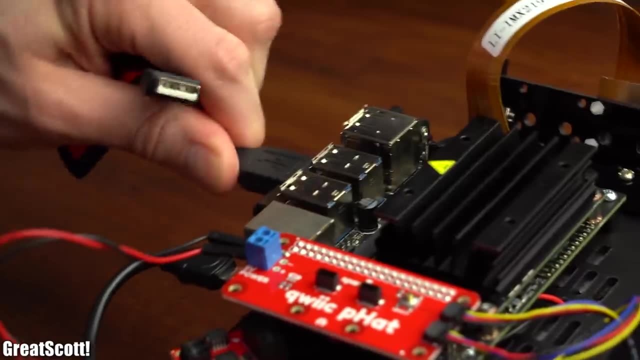 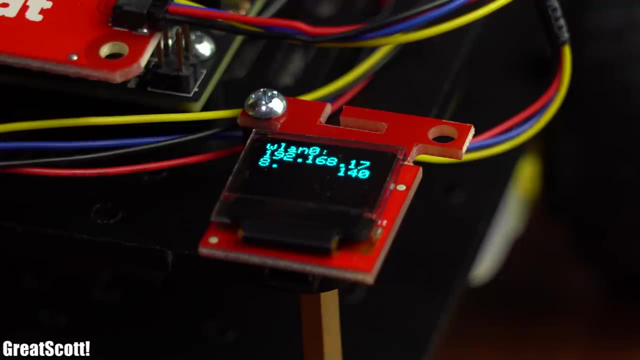 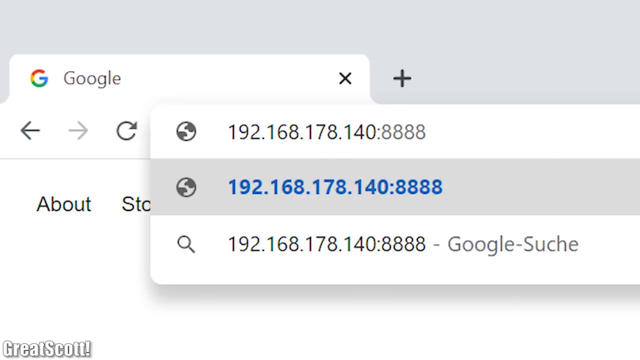 in order to connect to my wireless network through the Ubuntu graphical user interface. As soon as that was done, I shut down the computer, disconnected all devices and plugged its power once again. in to see the IP address of the system in my network, By entering this IP address in a browser, while using the port 8888, we can enter the JetBot's 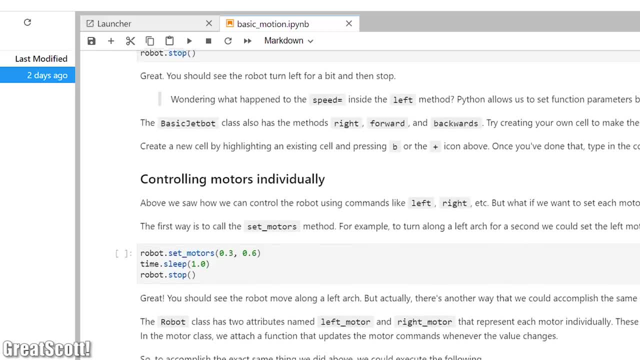 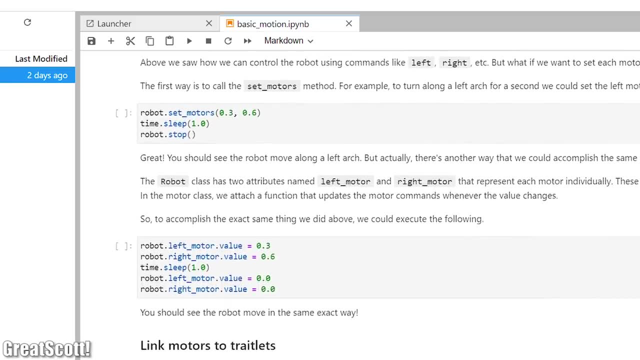 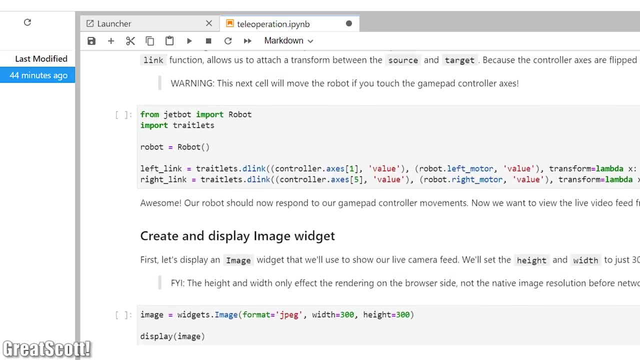 browser-based programming interface Which combines explanation, text code and graphics to give beginners a real easy entry when it comes to using this robot. And when I say easy, I mean the beginner's tutorials like basic motion and teleoperation, But when it later comes to collision avoidance and thus deep learning and AI. 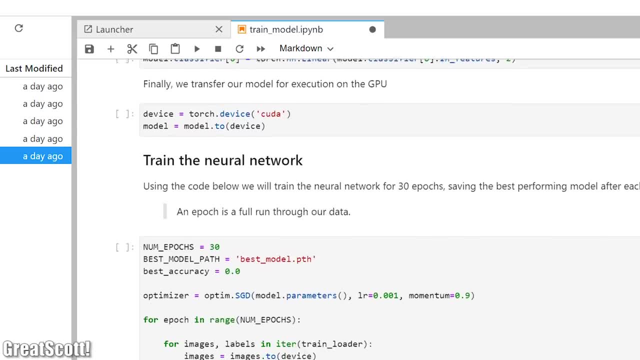 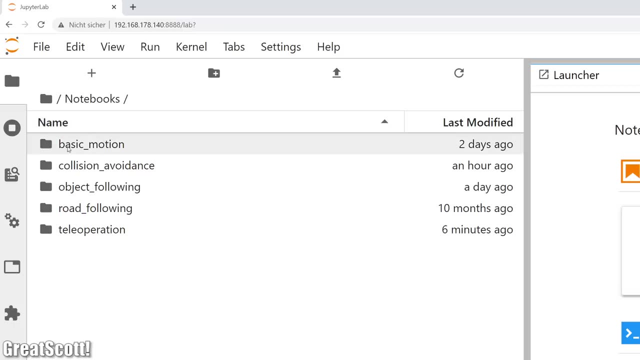 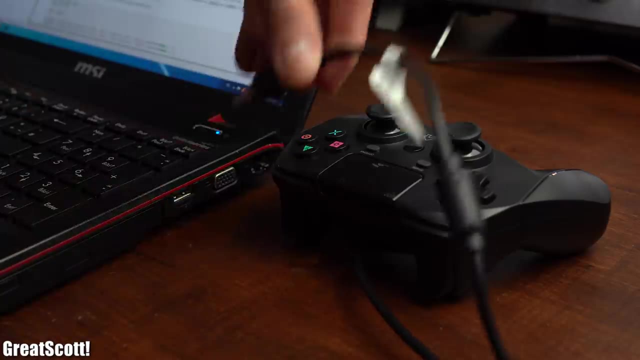 I was rather happy that those guides already existed, because I doubt that I could have ever used the AI. But anyway, I skipped the basic motion guide and went straight to the teleoperation example. There I plugged a gamepad into my computer and connected it with the software in order. 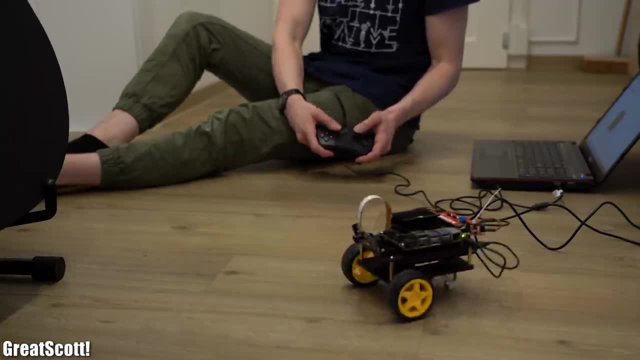 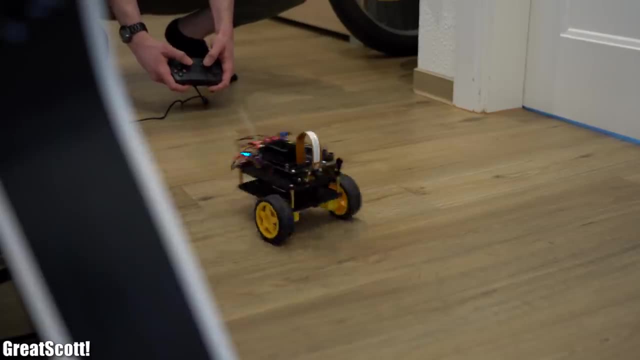 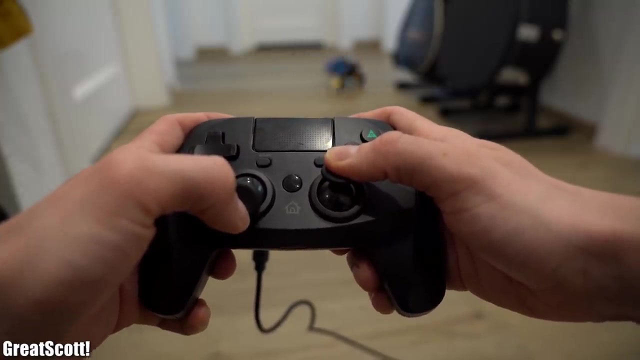 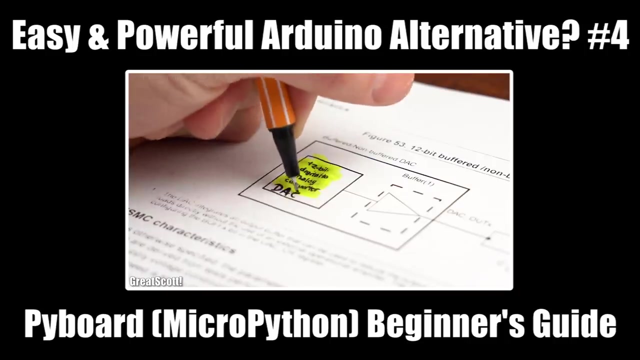 to remotely control the robot while also seeing a live feed of its camera input. This example basically told me that I assembled the robot correctly, and it also explained me how to do simple programming, for the robot functions through Python, which is a programming language that is also used by the Raspberry Pi. I even created a kind of video about it while trying. 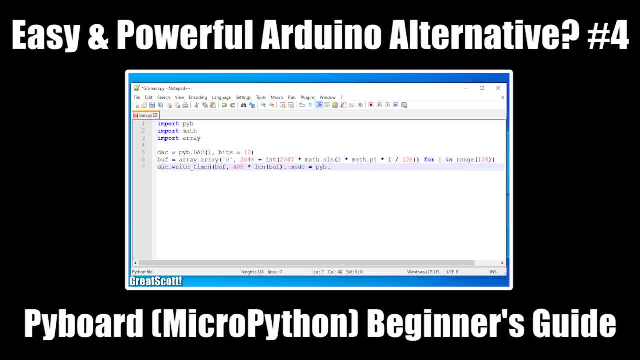 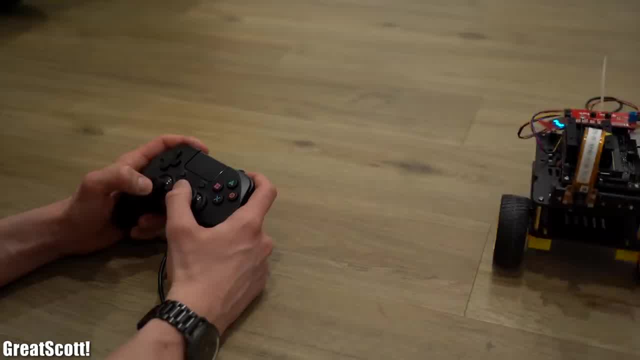 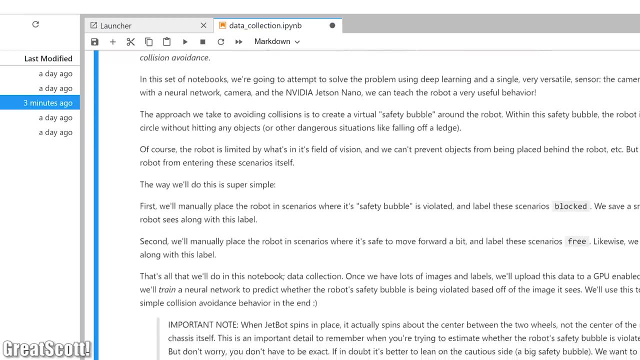 out a microcontroller that uses MicroPython, so feel free to watch that if you have no idea how Python works. But anyway, even though this example was fun, I wanted to move on to the AI part And, after reading through the three given guides, I had an idea of what was going on. 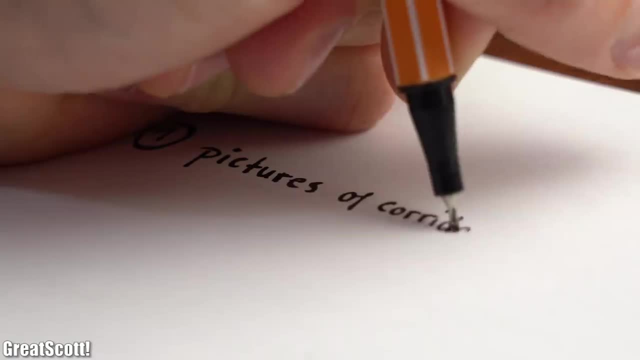 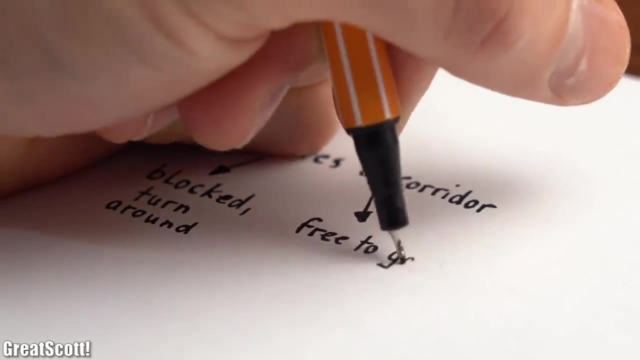 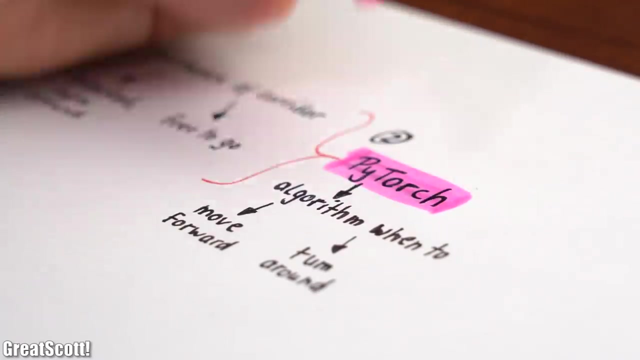 First off, I needed to take lots of pictures of where I wanted the robot to drive around, which I would have to classify as either blocked. so turn around or free to go. With the help of this database and the PyTorch software, the computer then creates an algorithm.